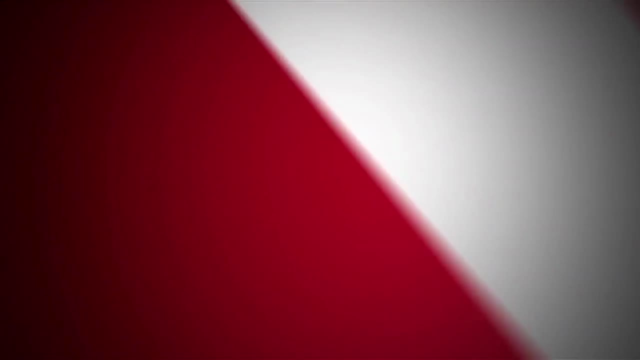 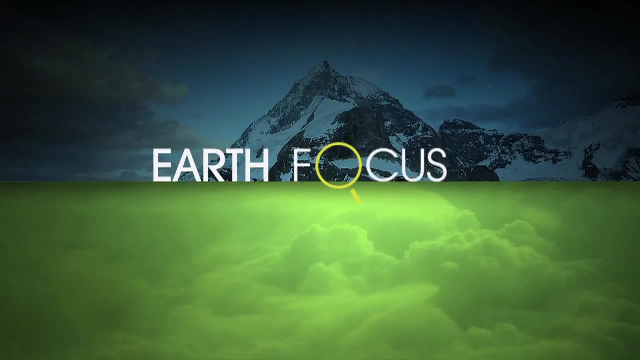 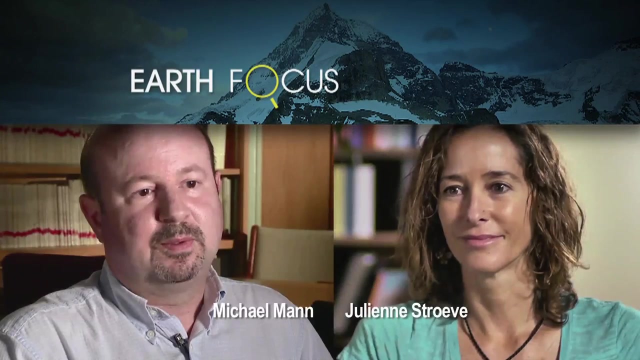 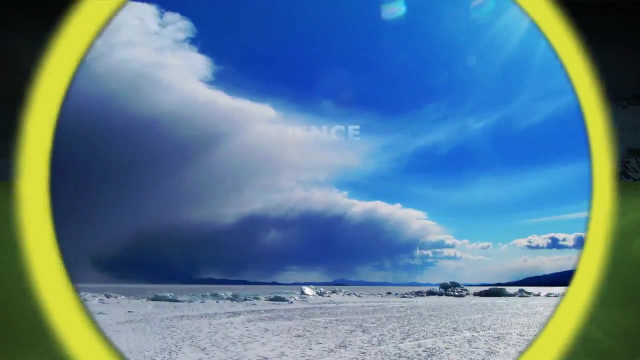 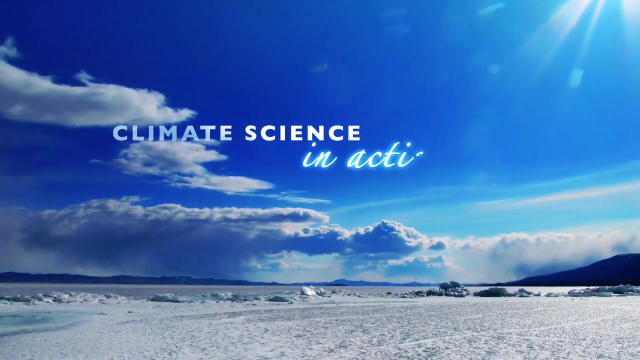 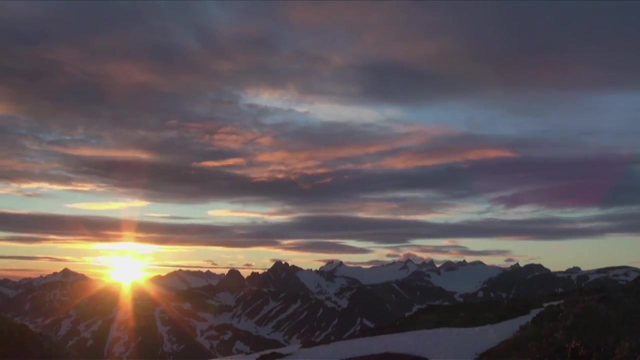 Today on Earth Focus From monitoring glacier melt and Arctic sea ice to what scientists say climate change may mean for our future. Coming up on Earth Focus On the edge of the Gulf of Alaska, straddling the icy border with Canada in the Coast Range. 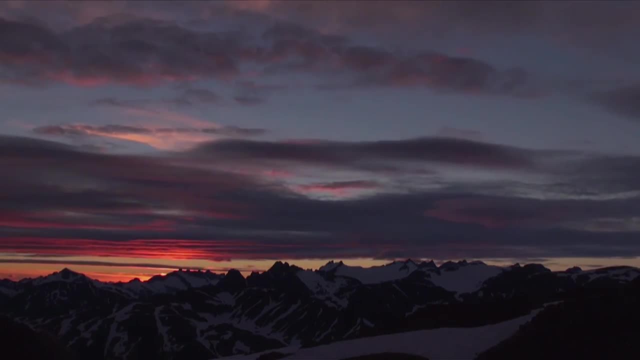 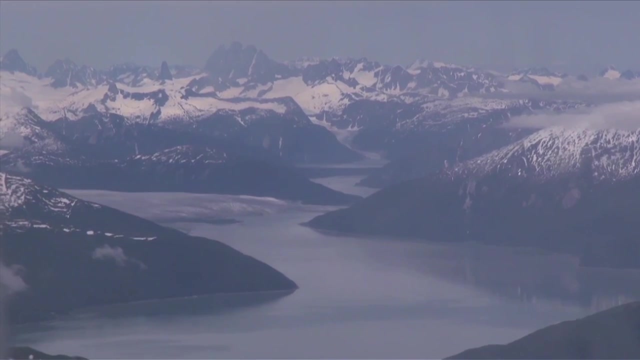 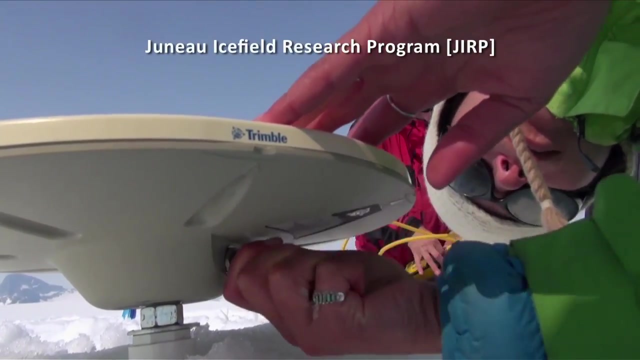 Mountains lies the Juneau Icefield. This is the fifth largest expanse of ice covering the planet and is the source area for hundreds of glaciers. The Juneau Icefield Research Program is a project of the US Department of Health and Human Services. The program, or JIRP, has been studying these mighty rivers of ice since 1946. 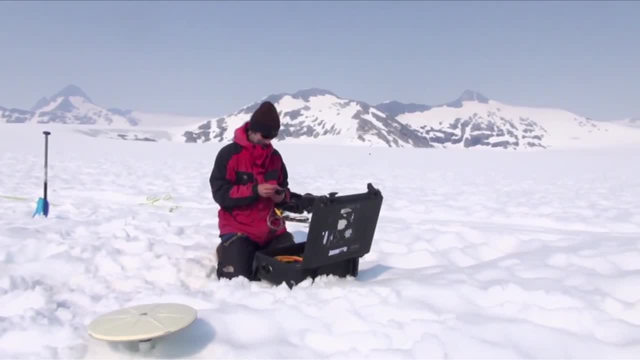 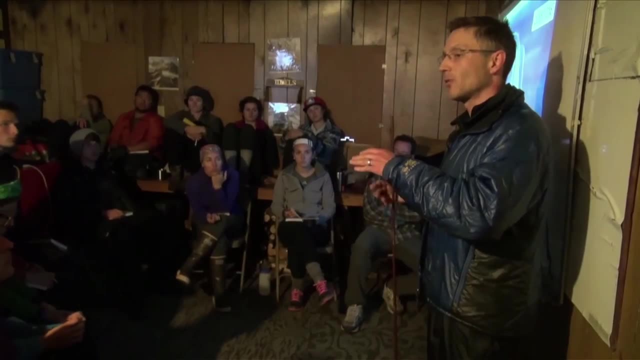 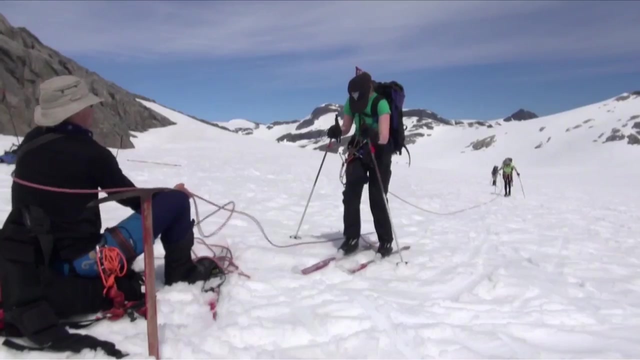 to better understand how our planet's natural environments are changing and what this means to our common future. There's a little bit of complexity as to why we use glacier ice. I came here as a science student 23 years ago and returned to work here this summer. 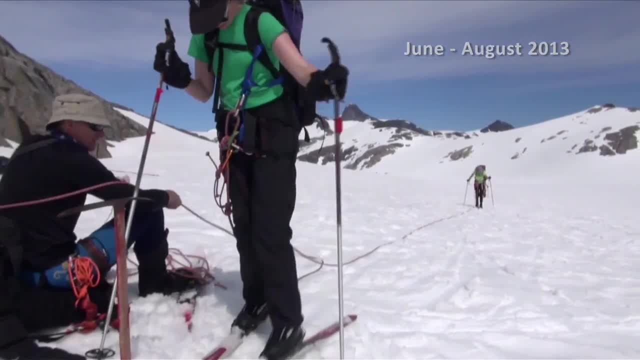 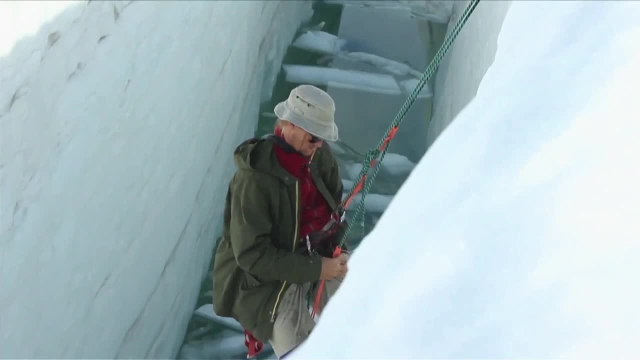 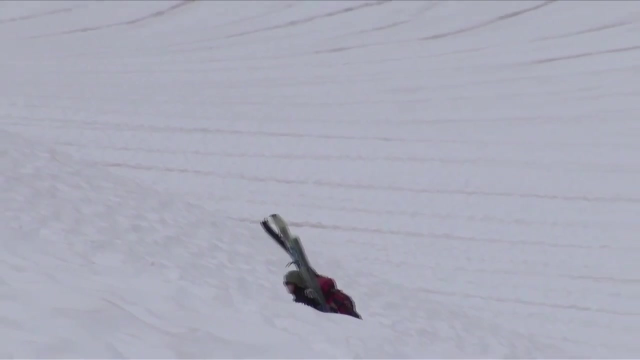 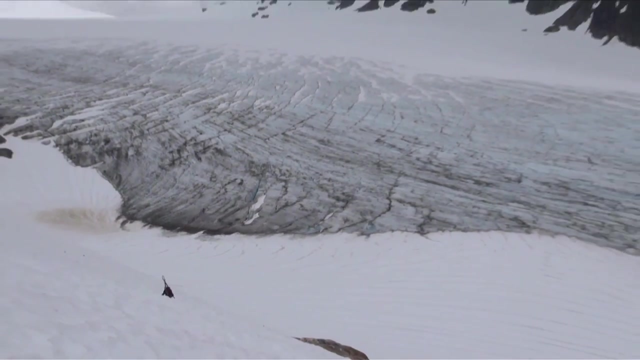 as a part-time staff member, Like other JIRPers, as we call ourselves. this project launched my interest in the natural world and continues to inspire my science reporting. Each year, a group of science researchers crosses this vast area, like I did, getting a chance to learn how to survive and conduct. 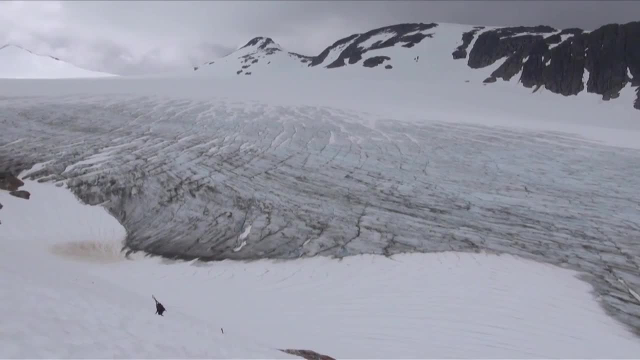 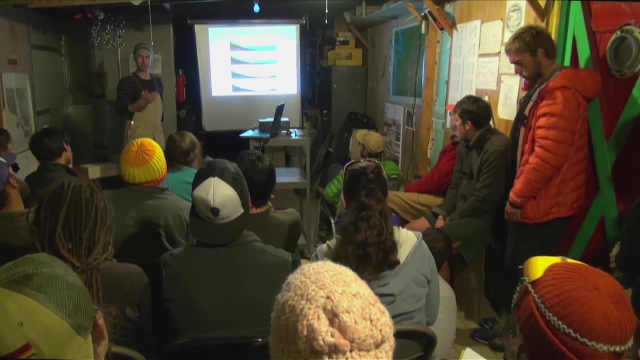 research in this, one of the most wild classrooms in North America, Supported and staffed by the Foundation for Glacier and Water Resources. this project is just a practice and conducted research in this one of the most wild classrooms in North America, Staffed by the Foundation for Glacier and Environmental Research, the Juneau Icefield. 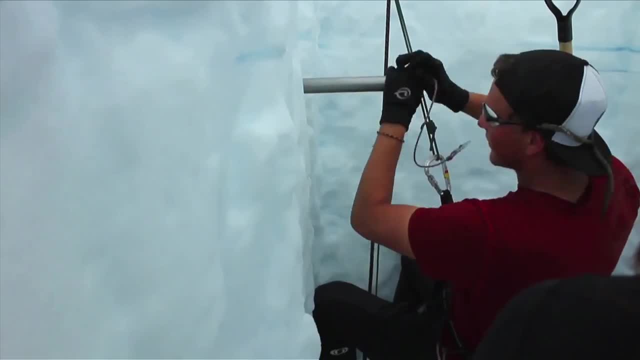 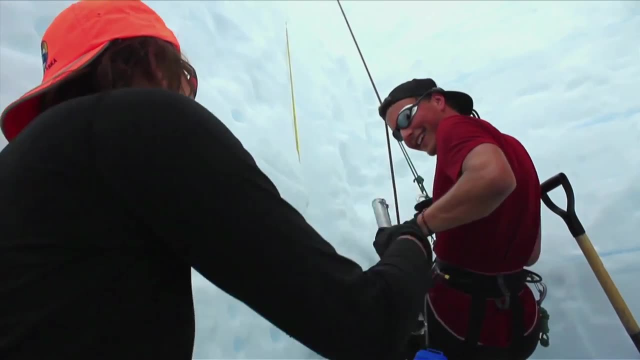 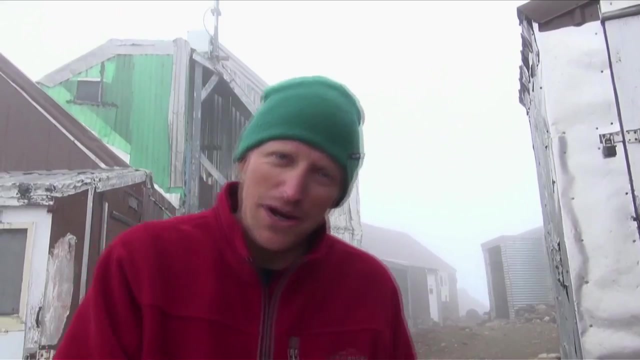 Research Program has some of the longest running glacial climate records in the world and is a treasure trove of valuable data about how our world's climate is changing. I'm here at Camp 17 on the Juneau Icefield and I'm going in to have a quick word with 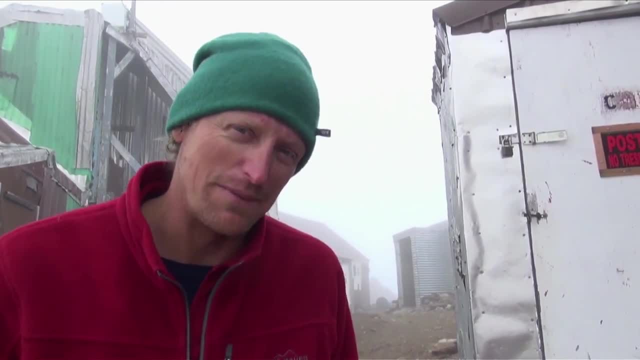 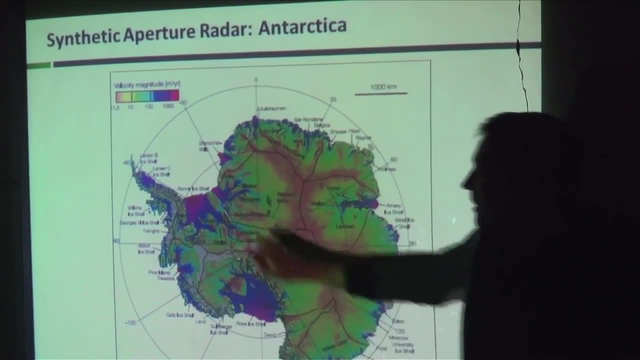 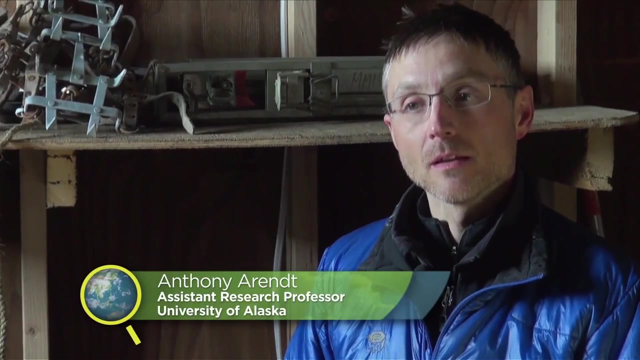 Dr Anthony Art. He's from the University of Alaska in Fairbanks and he's one of the guys who designed the latest satellite imagery systems for NASA to understand the mass balance of this. icefield. Glaciers respond immediately to any changes in climate. 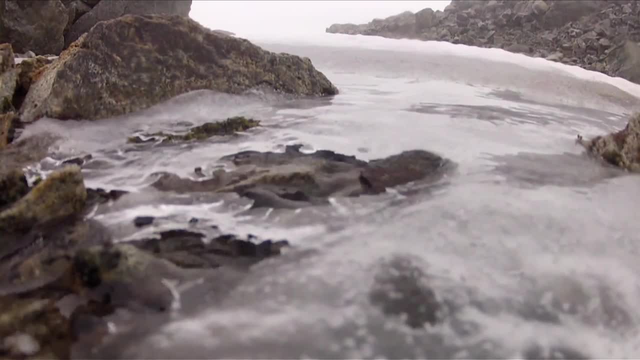 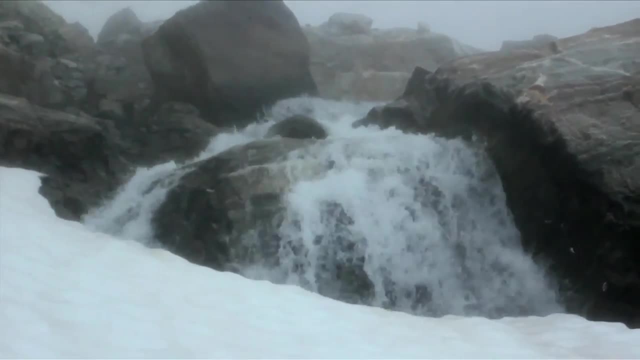 Their variations and their mass are determined directly by how much snow falls on them in the wintertime and how much ice and snow melts away due to warmer temperatures in the summertime. So by monitoring glacier variations we can understand a lot about climate systems, and 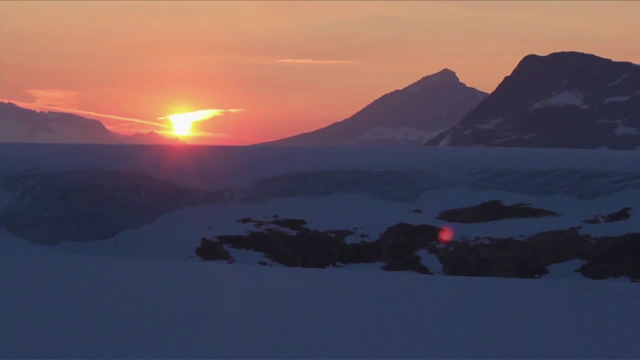 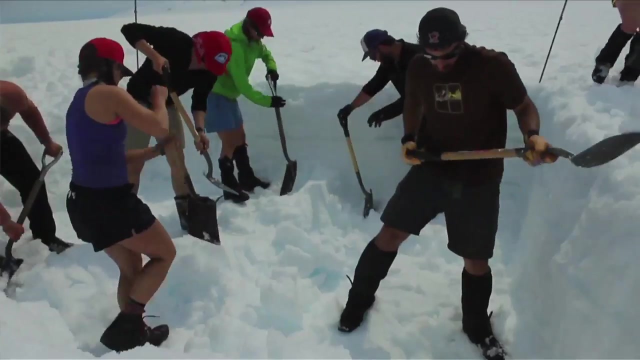 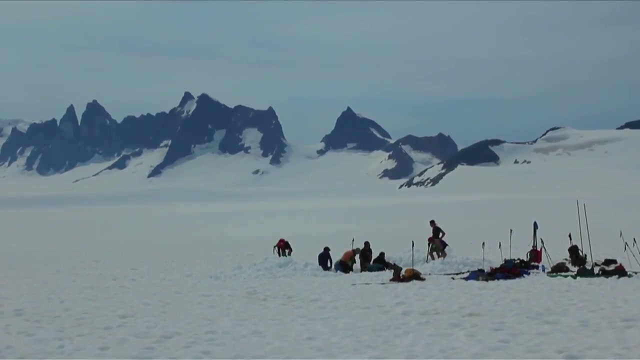 so they're One of the first sort of early hallmarks of climate change on the planet. Dr Art helps create high-resolution computer models of glaciers like this one, using data from satellites, airplanes and deep snow pits like these to develop a clear picture. 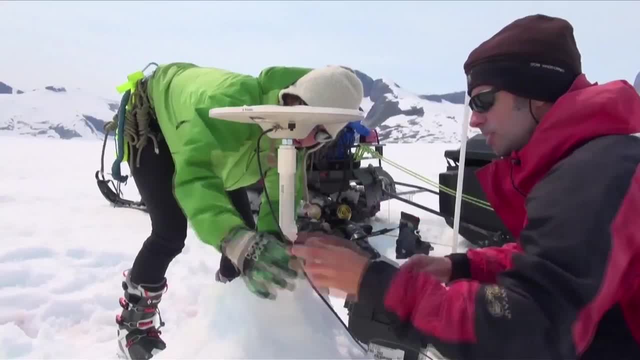 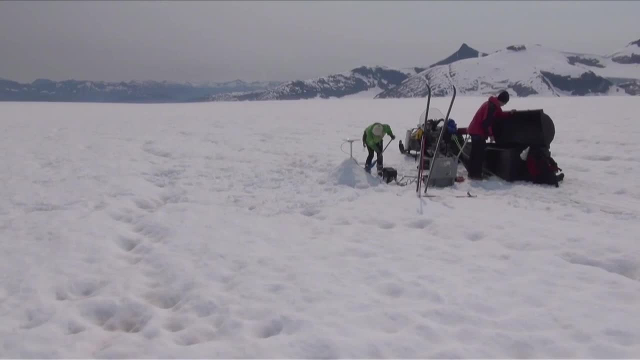 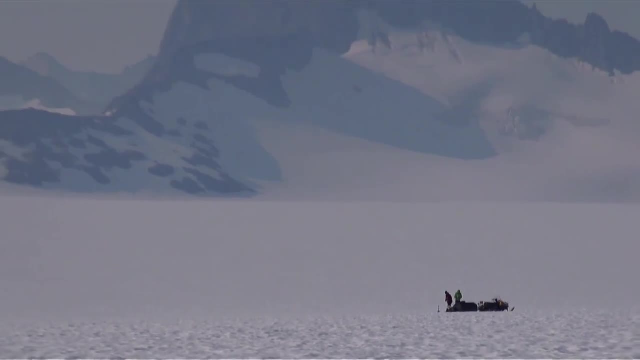 of our future global climate. Ninety-five percent of Alaskan glaciers are melting at an unnatural and unprecedented pace. We want to be able to quantify how much water is coming out of these systems every year and then use that information to develop models and predict in the future to help policy makers. 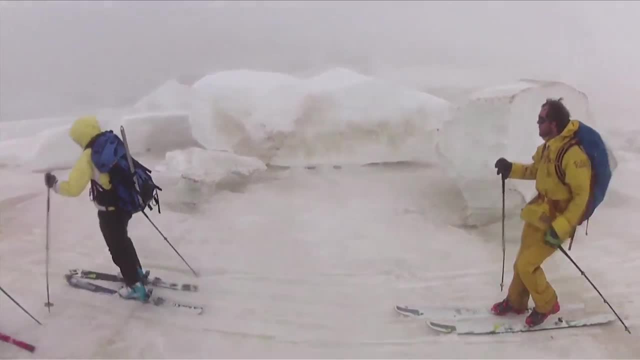 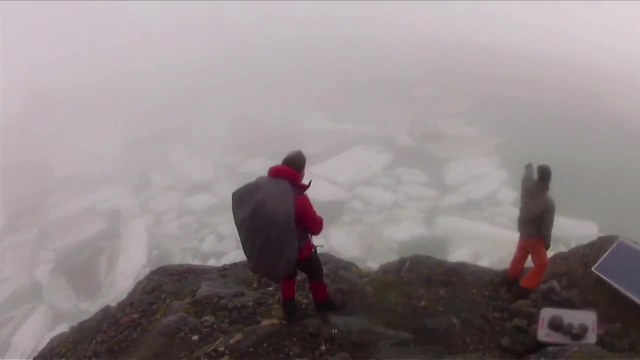 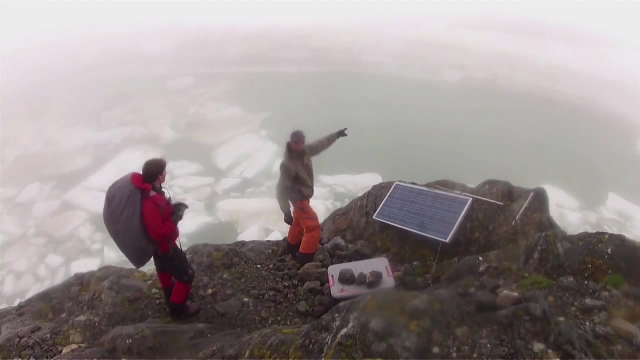 plan for potential effects of sea level change in the next fifty or a hundred years. Scientists like Dr Art come here to conduct research and to share their experience with the young and upcoming researchers taking part in the program. To collect the ground data that sophisticated scientists have gathered, Dr Art and his team have been working together. 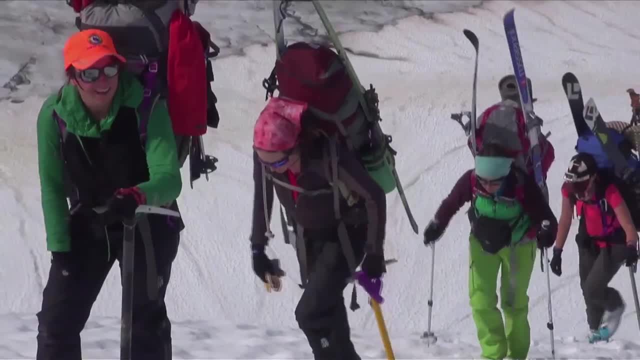 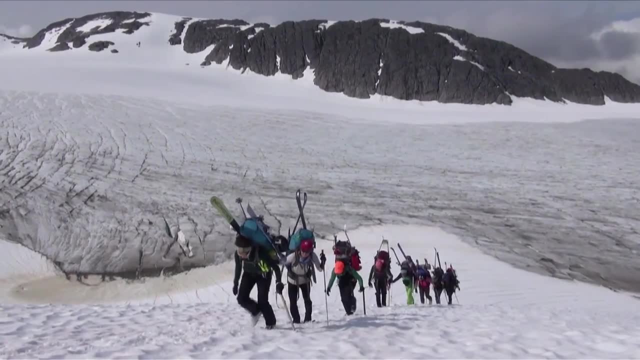 for over a decade. To get the data that sophisticated high-tech science depends on, students have to cross vast distances through the isolated heart of the ice field. In order to traverse the ice field safely, we train them extensively for the dangers of this rugged field experience. 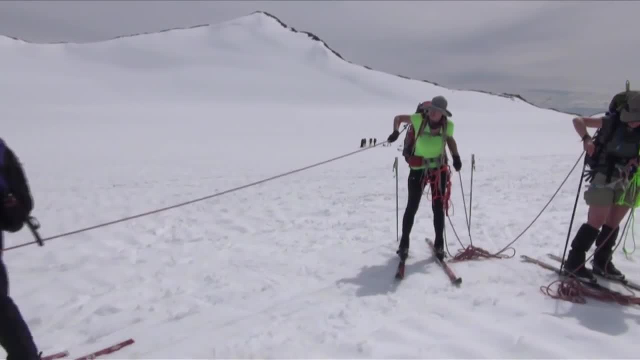 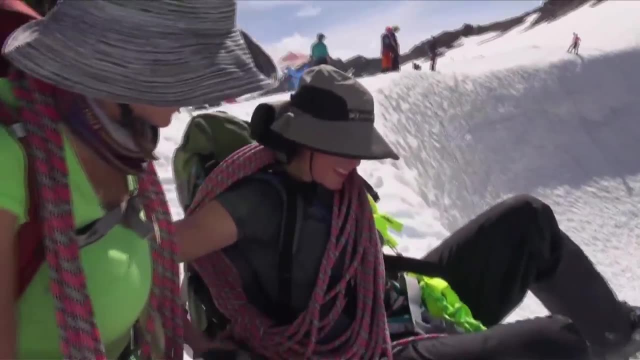 Here at Camp 17,. they learn adventure skiing, safe glacier travel on a rope and how to rescue a colleague from a crevasse. The training equips and inspires these students to learn more about the science behind the technology and how to use it. 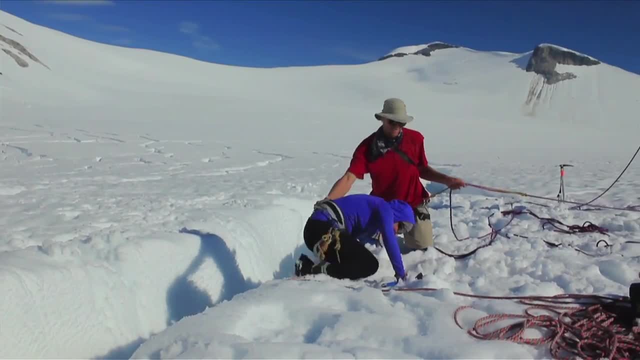 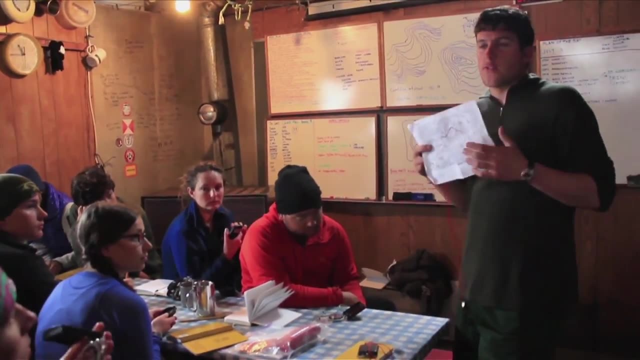 Dr Art is a graduate student at the University of Colorado, and he is a graduate student for a career in extreme environmental research, collecting data that the global scientific community depends upon to further the understanding of our changing world. This is just a useful tool in itself. 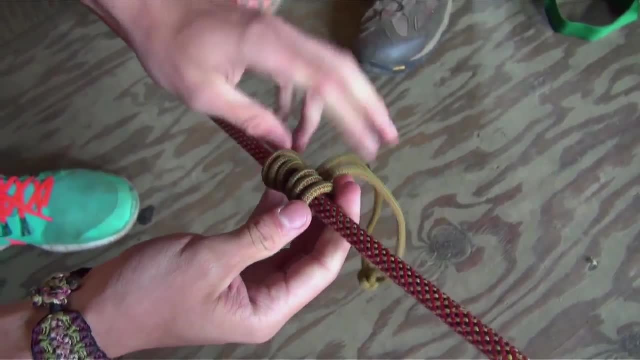 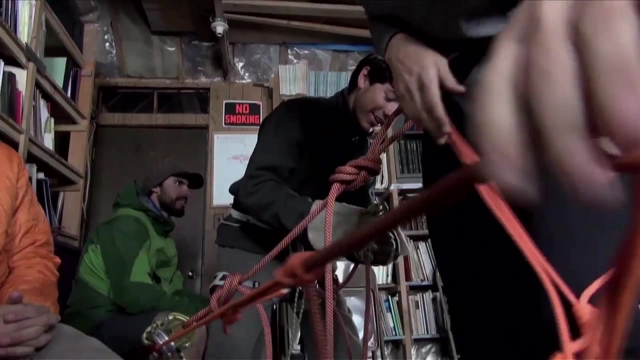 First off, we practiced tying knots. That was like the basis of all this- And then from those knots then we learned different ways to use the knots on a rope, which then you learned how to ski with a rope team and what to do in case something bad happens on a rope. 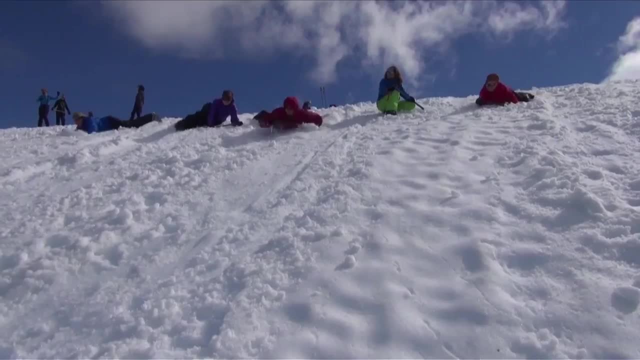 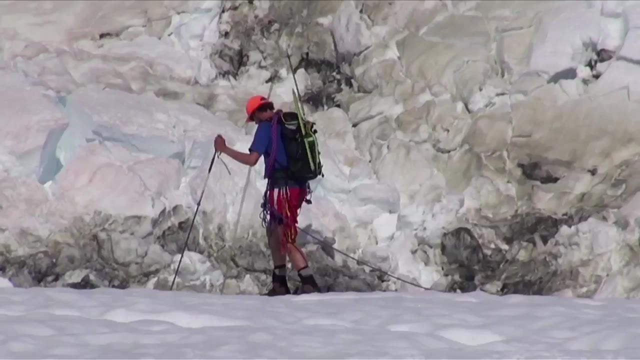 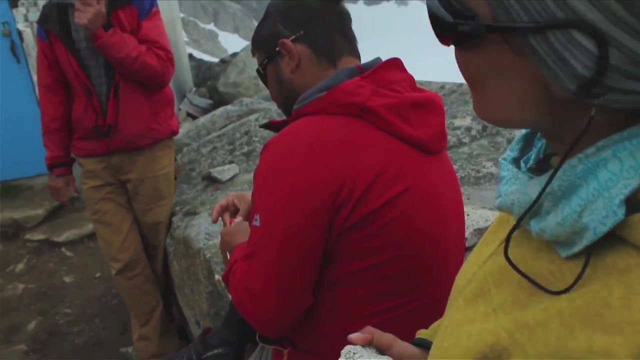 team like a fall into a crevasse and how to save a team member that has fallen. After science and safety training at Camp 17,, the participants start their traverse across the ice field doing field work in geology, glaciology, climate change and other. 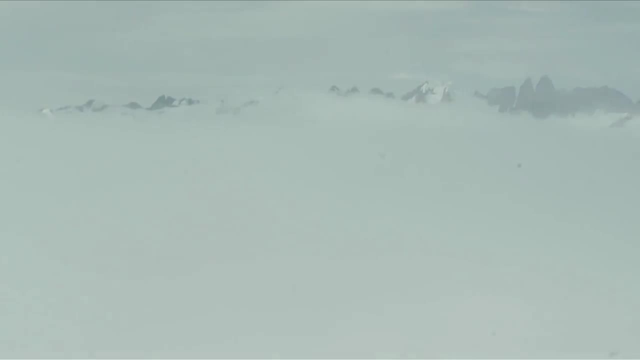 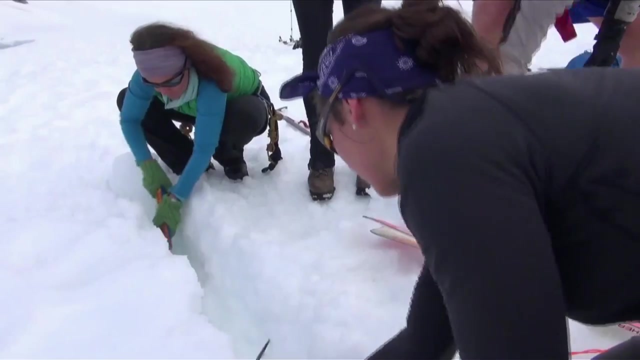 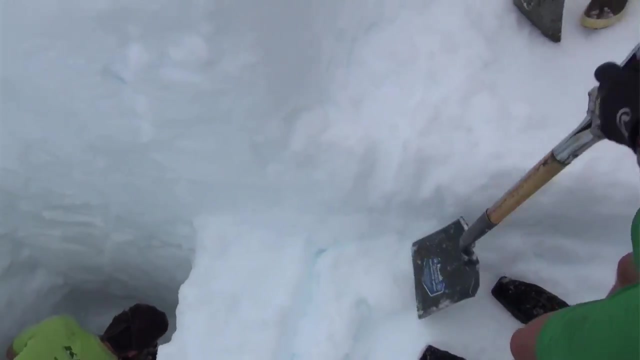 disciplines. When these people come onto the ice field and experience the glacial environment by making measurements, they can see how that ecosystem is changing this year and in years before. To be on the Juneau ice field is a fantastic experience for me. I'm part of a major program. 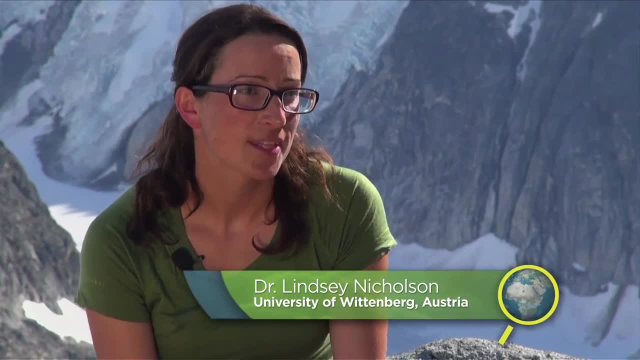 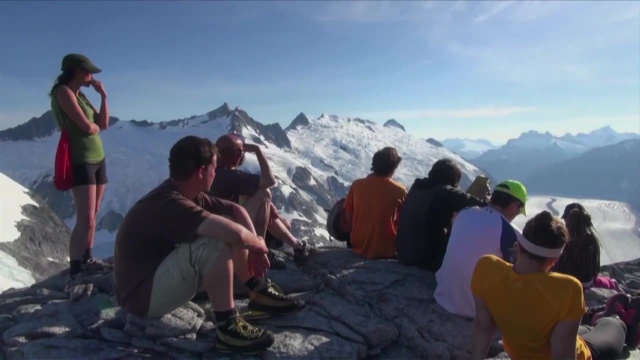 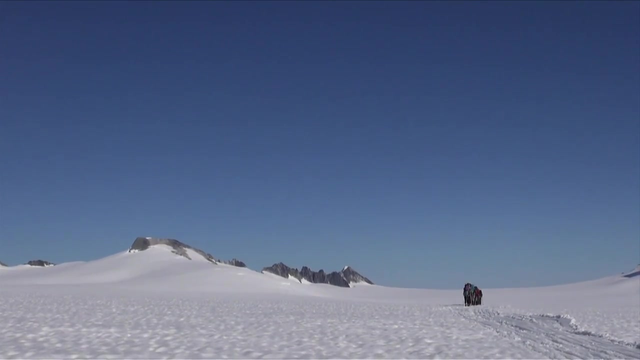 that monitors mass balance of an important glacier and in addition it gives me the opportunity to try and contribute to the scientific development of young scientists. Mass balance indicates the health of a glacier. A positive mass balance means that the glacier is growing. A negative mass balance means that it is shrinking. 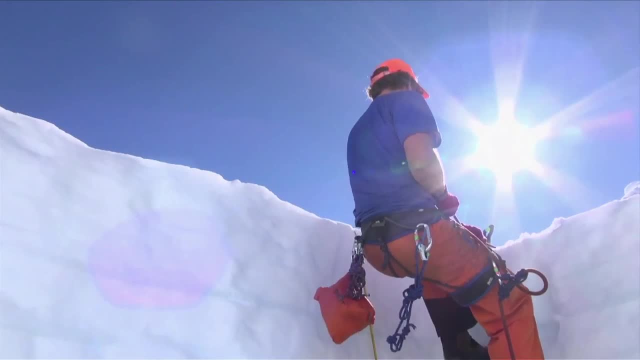 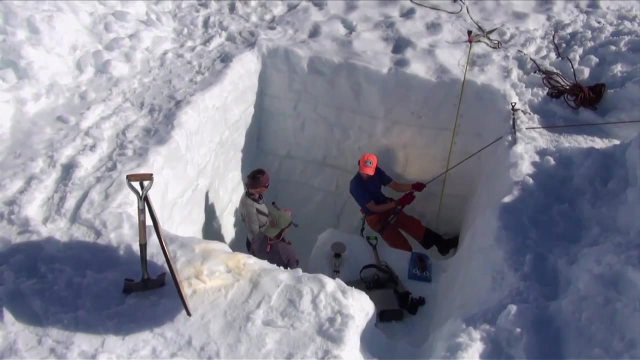 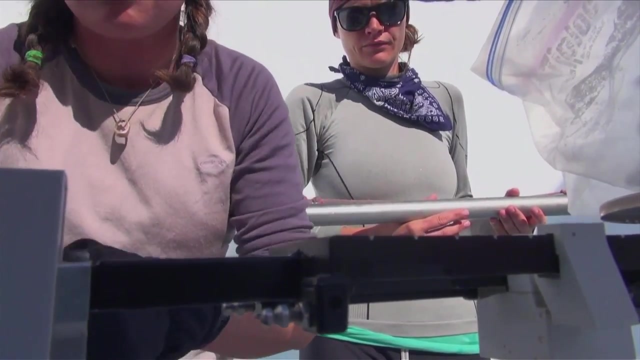 The older a mass balance record is, the more valuable it becomes. Long-running studies provide a historical average against which this year's data can be compared, showing how the climate has changed and what may happen in the future. The mass balance data that's been collected by the JERC program is an extremely important 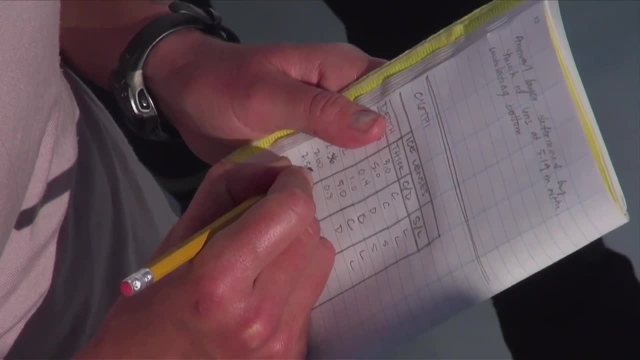 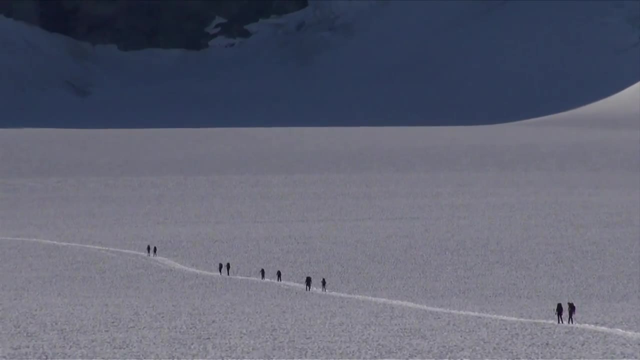 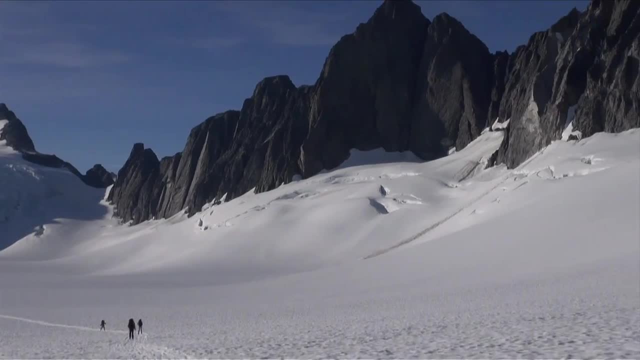 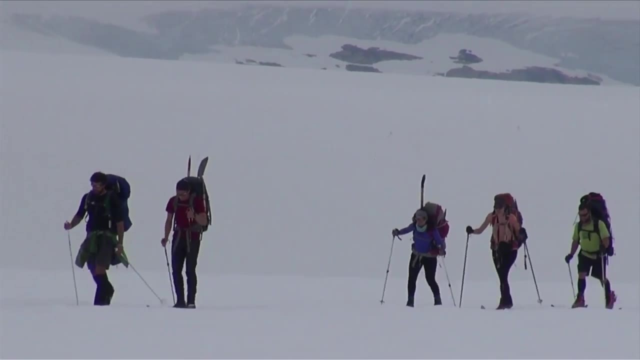 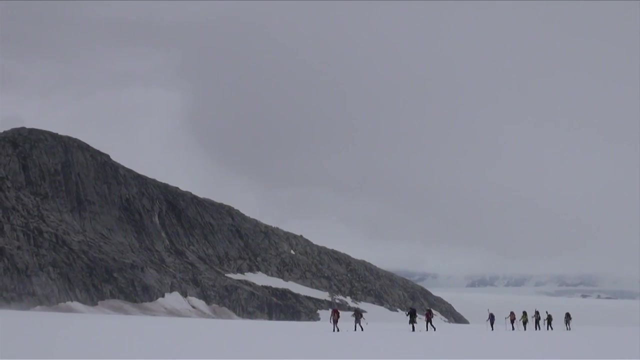 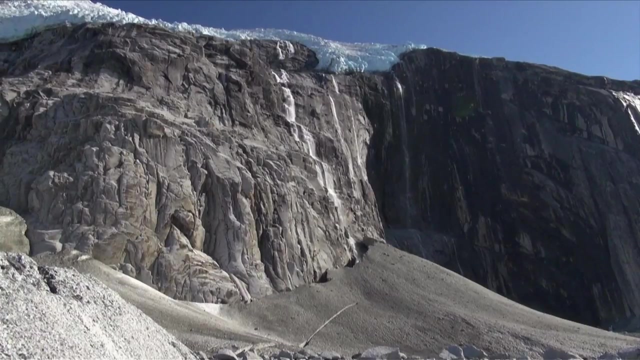 It's a lot, It's a lot, It's a lot. You're talking about 100,000. Keep Kalimantan years, which would increase the size ofhes ofts a glacier in 10 years. The relative amounts of snow fall and melt represent this mass balance. A positive managers. 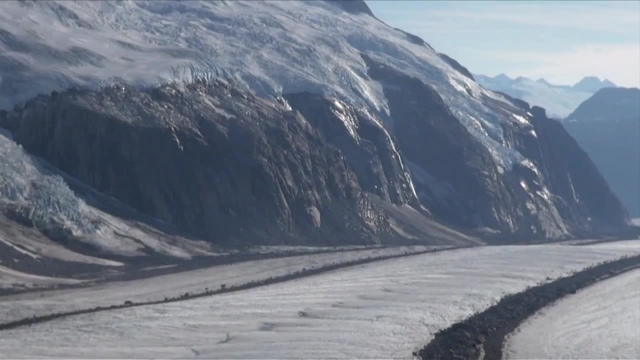 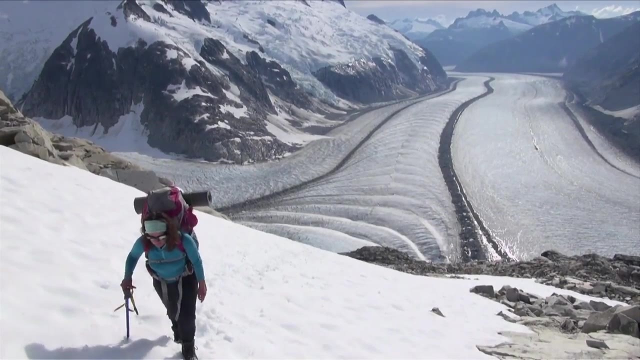 bank accounts. a positive mass balance indicates that the glacier is growing. On the flip side, if the Glacier has less snow fall and more melt, the glacier becomes smaller. So how have estimation of the health of this 3,900 square kilometer ice sheet? 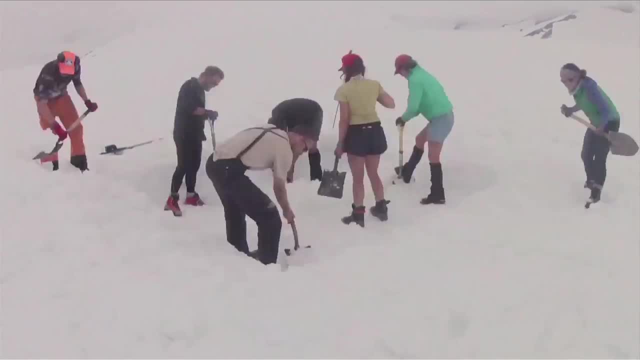 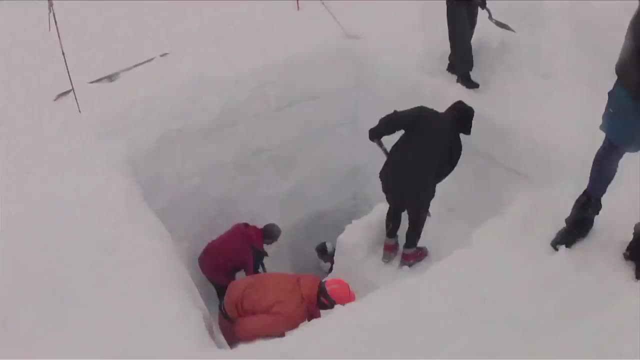 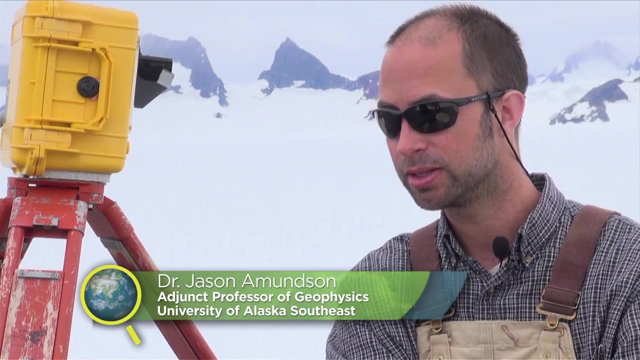 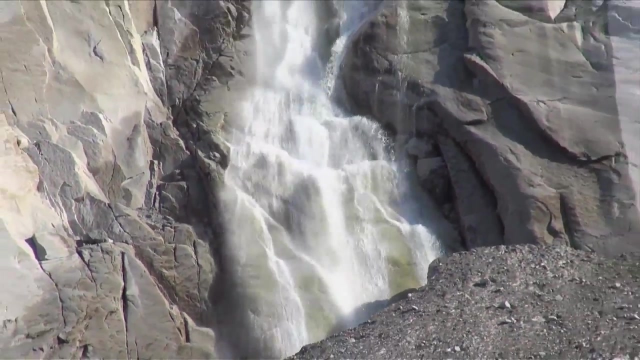 They dig a lot. By digging many pits like these, scientists, like Dr Jason Amundsen, calculate how much melted ice is flowing into the ocean When the glaciers or ice sheets retreat. one thing they do is they contribute to sea level rise, but they also affect atmospheric circulation patterns, which propagates downstream and affects 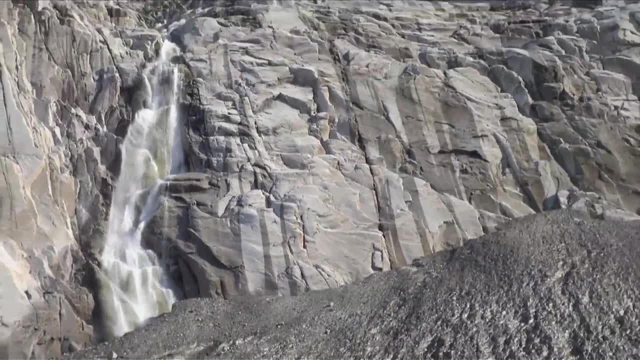 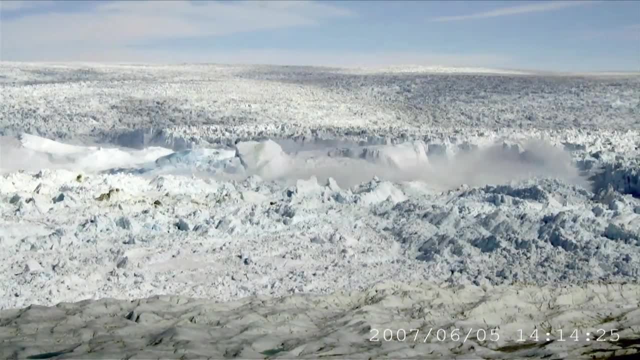 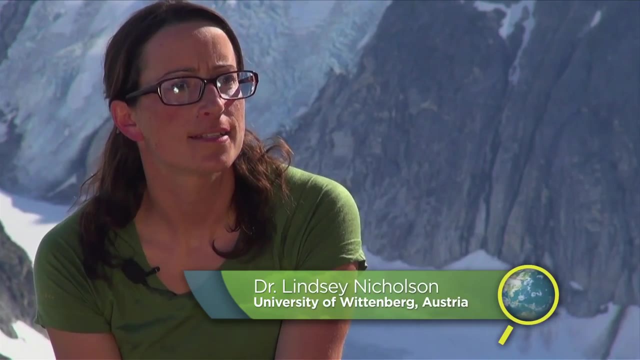 other things. There will be changes in amount of freshwater runoff into the ocean which will affect the ocean properties, which could affect the marine life. The global sea level is going to rise and it will rise by varying amounts depending on where you are in the world. 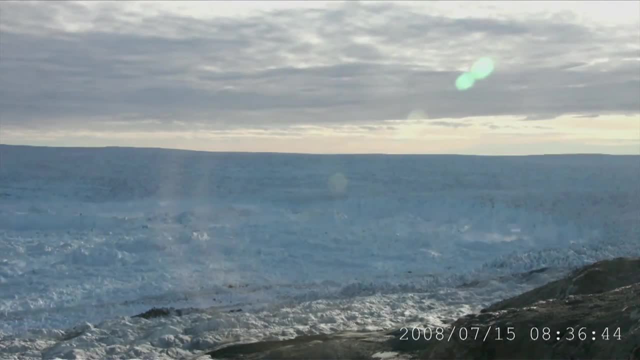 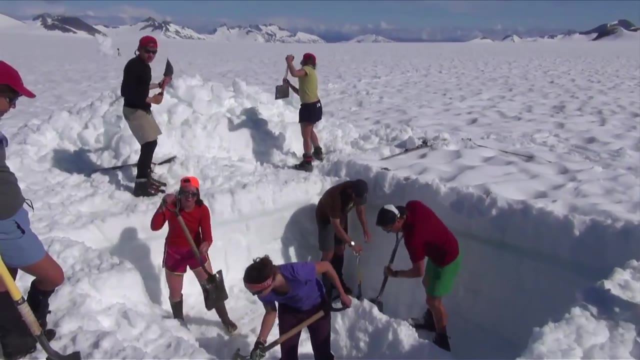 The contribution from glaciers DIGGING SNOWPITS HAS BEEN USEFUL FOR ALMOST 60 YEARS ON THE JUNO ICE FIELD BUT WHEN THESE SNOWPITS ARE PAIRED WITH NEW GROUND-BREAKING TECHNOLOGIES, THE SCIENCE 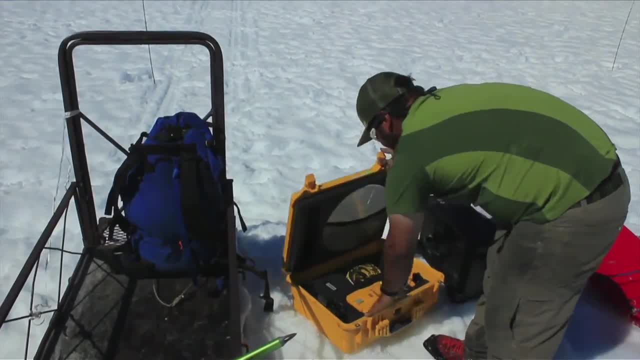 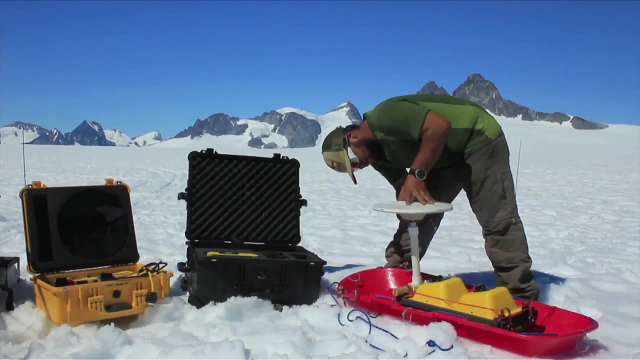 BECOMES EVEN MORE SUCCESSFUL. SALVATORE CANDELLA IS USING A POWERFUL GROUND-PENETRATING RADAR- OR GPR AS IT'S KNOWN- TO GET INFORMATION FROM THE VAST AREAS BETWEEN SNOWPITS, USING THE PITS THEMSELVES AS A REFERENCE. 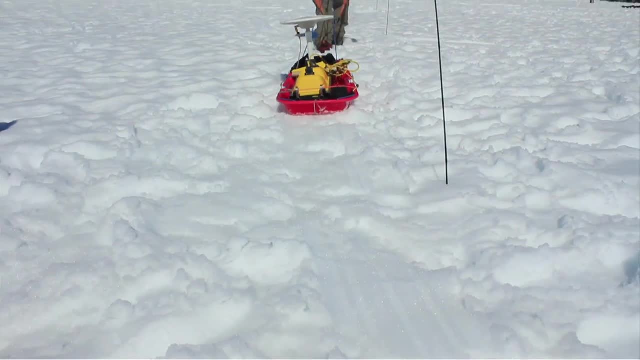 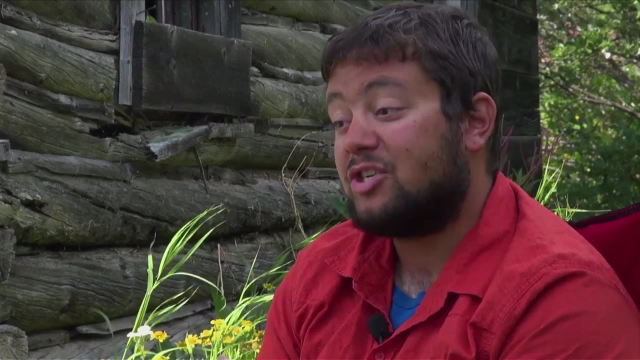 THE DIGGING OF PITS AND USING GROUND-PENETRATING RADAR REALLY TIES WELL TOGETHER, SINCE I'M IMAGING WHAT'S IN THE GROUND AND THEY'RE ACTUALLY DIGGING IN THE AREA I'M IMAGING. 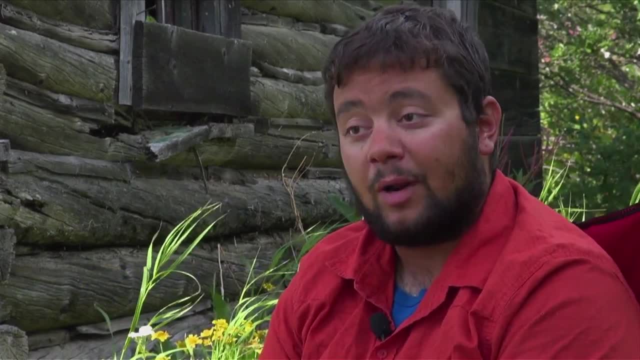 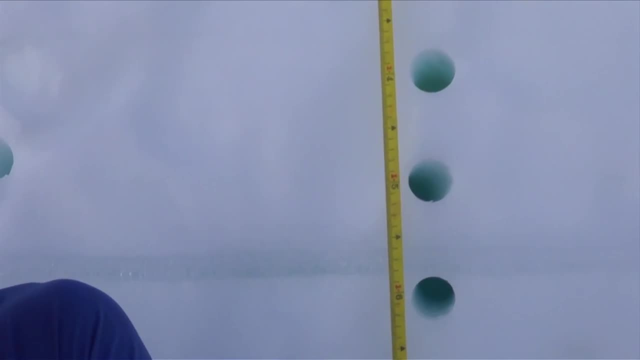 THEY COMPLIMENT EACH OTHER IN THAT IF I HAVE A QUESTION ABOUT WHAT I'M SEEING ON THE RADAR, I CAN GO JUMP IN A FIVE-METER DEEP HOLE AND ACTUALLY SEE WHAT IS THERE AND BY PAIRING THEIR VISUAL OBSERVATIONS WITH WHAT'S ON THE RADAR, IT ALLOWS US TO COME TO. 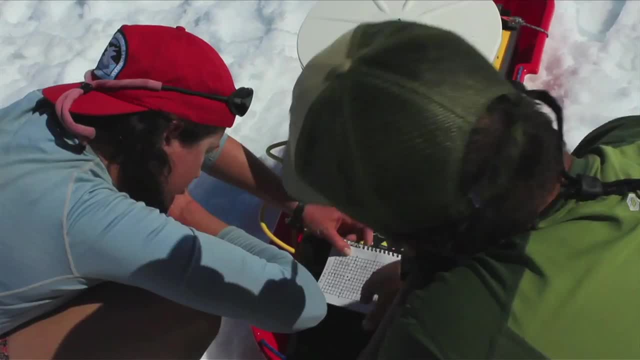 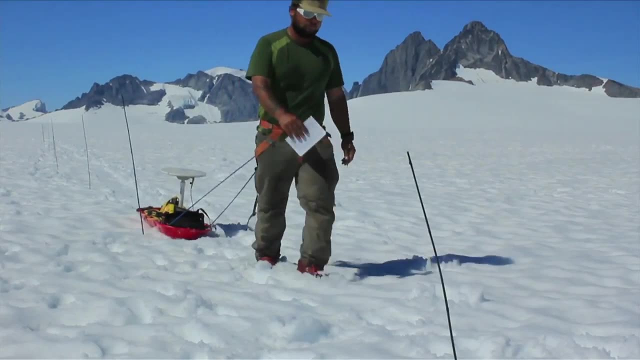 A MUCH DIFFERENT PERSPECTIVE. IT'S A MUCH STRONGER CONCLUSION ABOUT WHERE THE ANNUAL LAYER IS OR WHERE A SPECIFIC DENSITY CHANGE MIGHT BE THAT THEY'RE LOOKING FOR IN THE MASS BALANCE PROCESS. 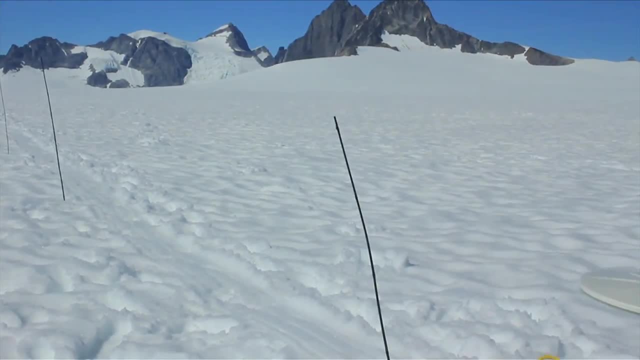 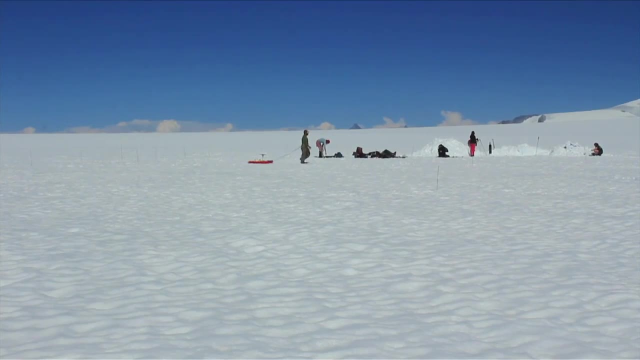 BY DRAGGING HIS GPR SLED, NAMED THE BUMBLE BEE, AND USING THE PITS TO CALIBRATE IT, CANDELLA IS HELPING CREATE A MUCH BETTER UNDERSTANDING OF THIS DYNAMIC GLACIAL SYSTEM. 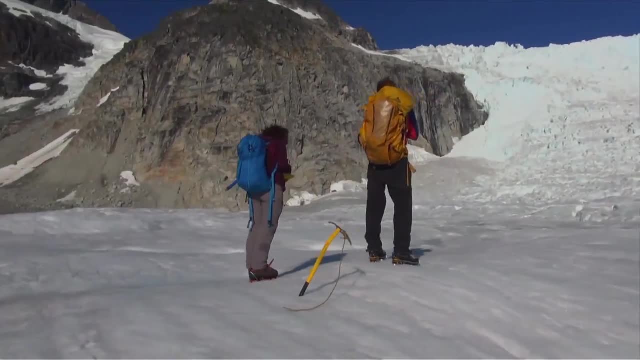 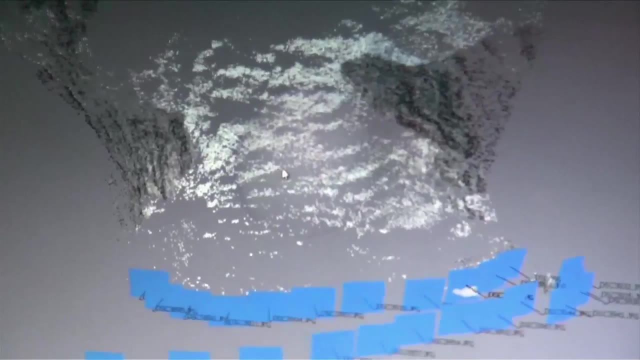 THE RESEARCHERS ALSO MAP THE MOVEMENT OF THE PITS. THEY'RE USING THEM TO DETERMINE THE MOVEMENT OF THE ICE WITH GPS AND 3-D IMAGERY. SO WE WERE SUCCESSFUL. I'D SAY WE WERE VERY SUCCESSFUL. 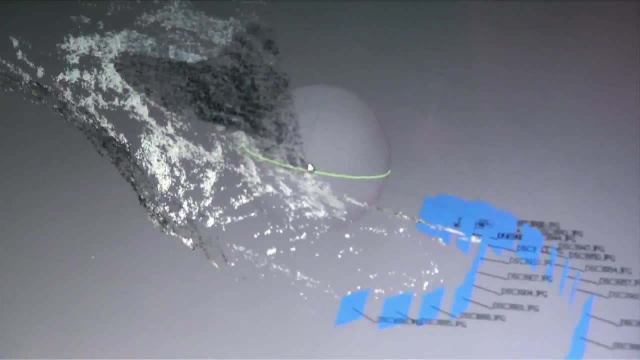 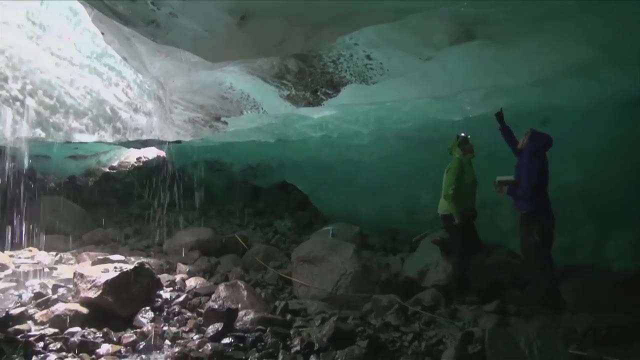 ROTATE IT AROUND, OKAY. SO I GRAB IT AND I JUST MOVE IT AROUND. WOW, THEY EVEN GET DEEP UNDER THE ICE IN VAST COMPLEXES OF SUBGLACIAL CAVERNS TO CALCULATE HOW THE 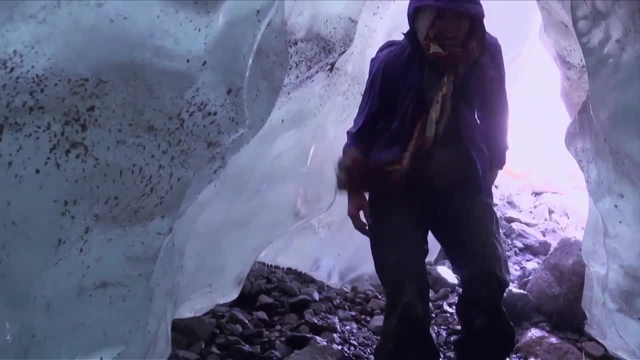 GLACIERS ARE MELTING FROM THE BOTTOM UP. THE HUGE LIEUWELEN GLACIER ENCAMPS THEM. THE HUGE LIEUWELEN GLACIER ENCAMPS THEM. THE HUGE LIEUWELEN GLACIER ENCAMPS THEM. 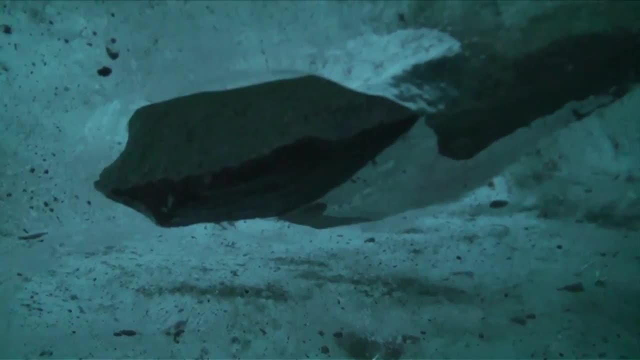 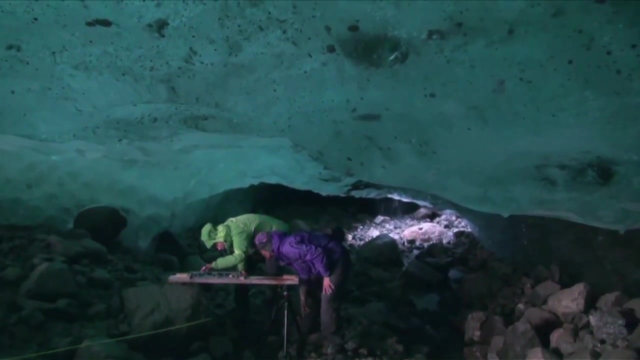 CANADA IS MELTING FAST EXPOSING MORE OF ITS SECRETS FOR RESEARCHERS: BROOKS, STAMPER AND MIRA DUTCHKA TO DISCOVER USING PHOTOGRAMMATRY AND ICE LENS MEASUREMENTS. 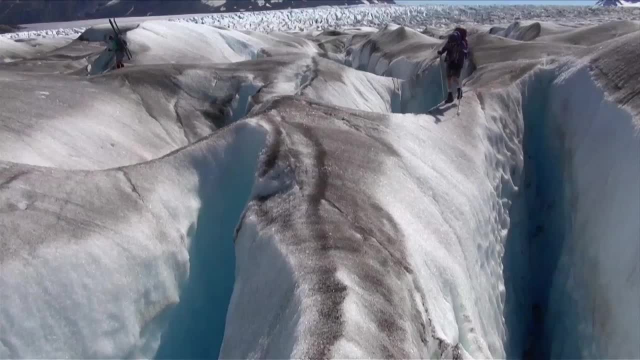 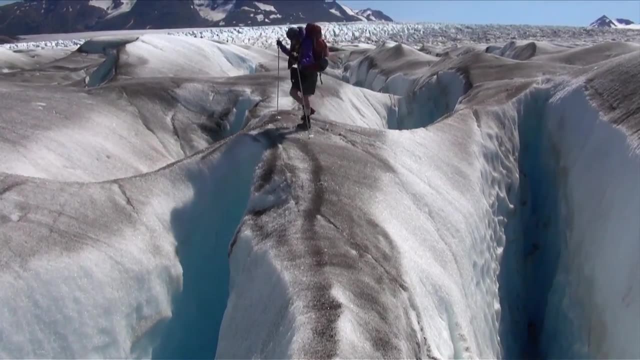 AS THE 2013 FIELD SEASON ON THE ICE FIELD COMES TO A CLOSE, WE MAKE OUR WAY NORTHEAST AND WALK OFF THE LIEUWELEN GLACIER THROUGH A DANGEROUS CREVASSE FIELD. WE'RE WINDING OUR WAY THROUGH THE CREVASSES OF THE LIEUWELEN GLACIER. 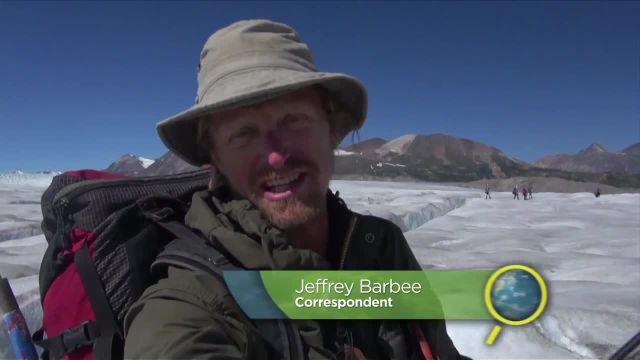 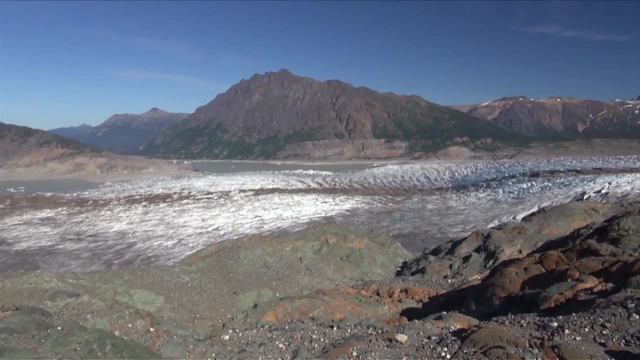 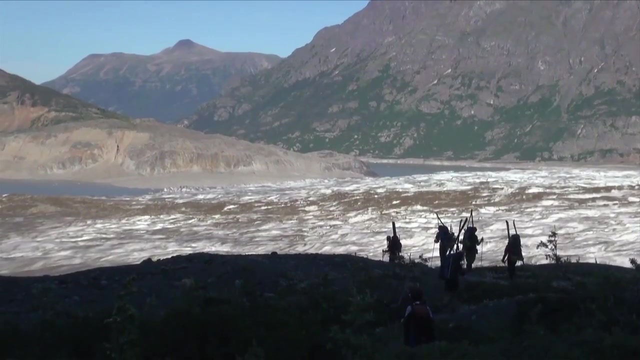 EVERYONE'S MAKING THEIR WAY VERY CAREFULLY HERE, because the glacier gets a little broken up. But it's a beautiful day and it looks like we might make it all the way to Lake Atlin. We struggle down through this dusty and blowing newly uncovered ground. 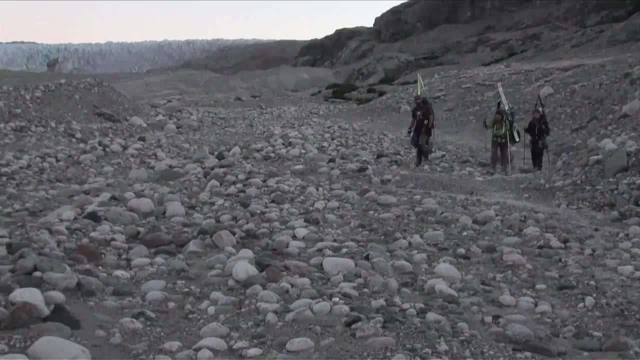 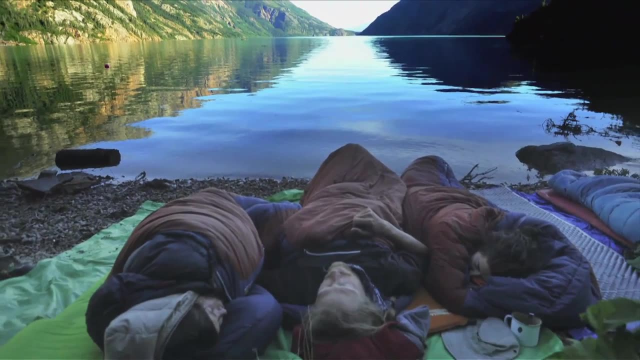 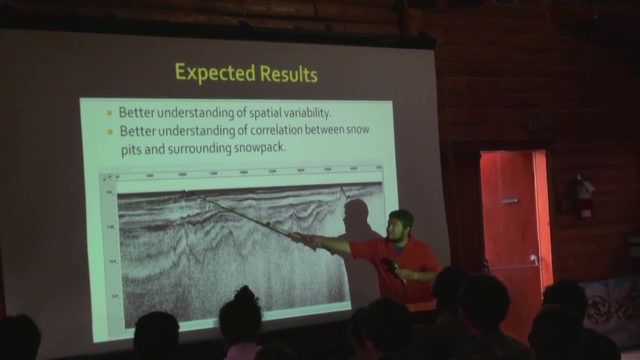 where the vast Llewellyn has melted. and finally we make our way down this long valley to Lake Atlin. Here we're picked up by a boat and start deciphering the data and working it into the scientific literature, where researchers around the world can use it to fine-tune their climate change predictions. 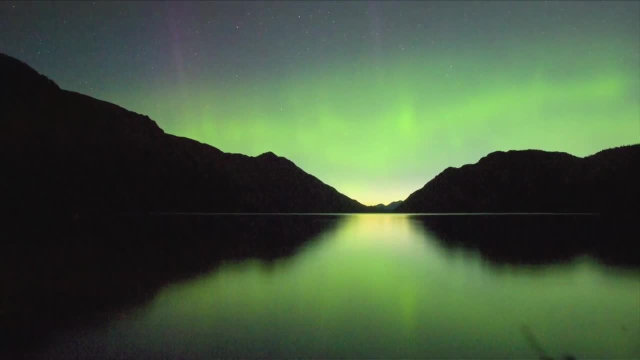 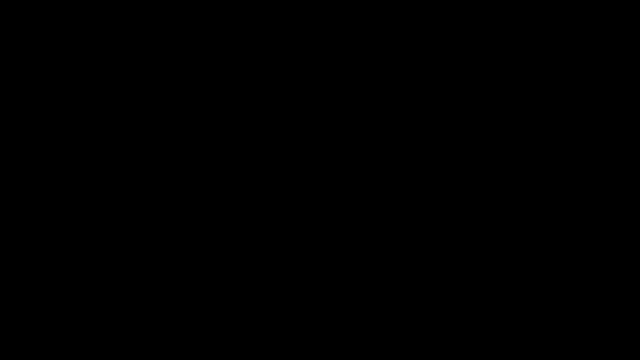 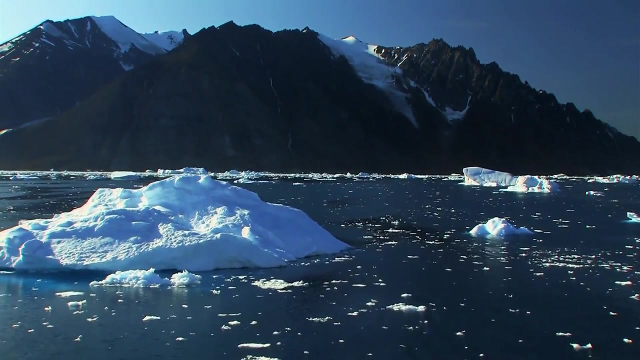 From the Glaciological and Arctic Sciences Institute on Lake Atlin, British Columbia. this is Jeffrey Barbee reporting for Link TV. Glaciers are not the only things melting, So is all Arctic sea ice. Just how fast is the sea ice melting? 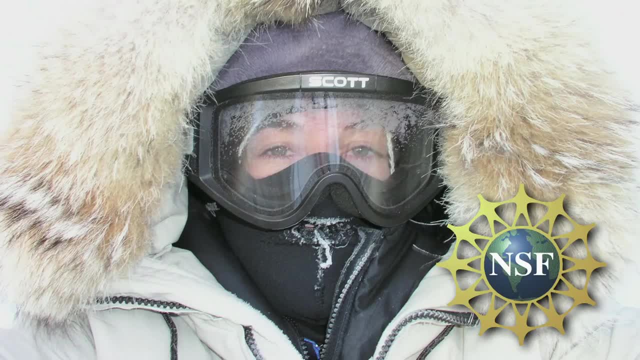 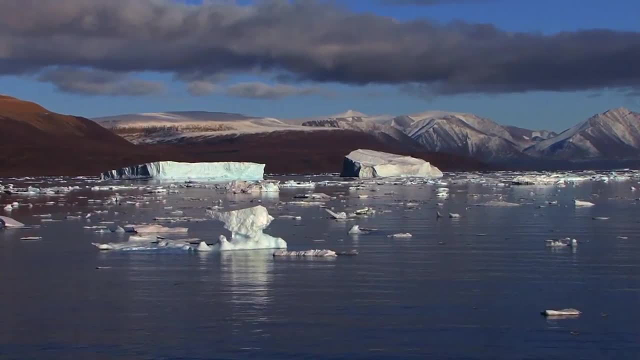 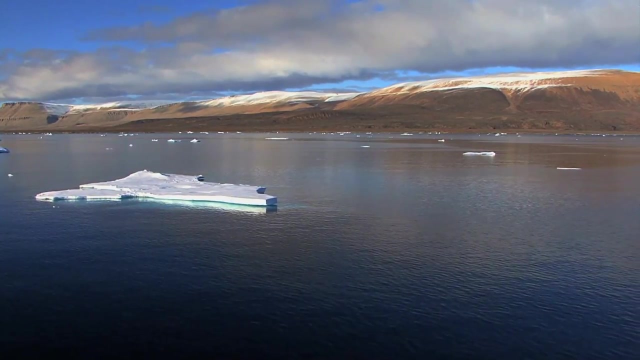 Research scientist, Julianne Struve, is working with the National Science Foundation to find out. You know, I knew the importance of snow and ice and helping regulate the planet's temperature, And it's one of the reasons I went into studying snow and ice. 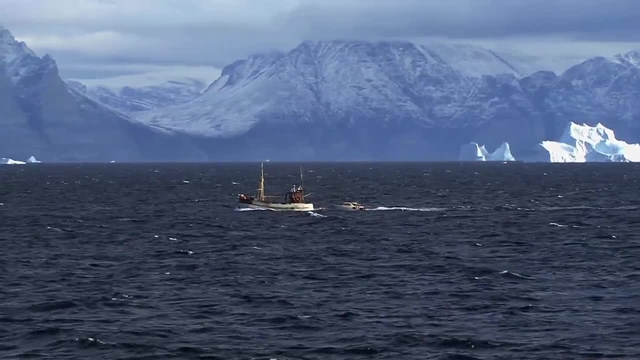 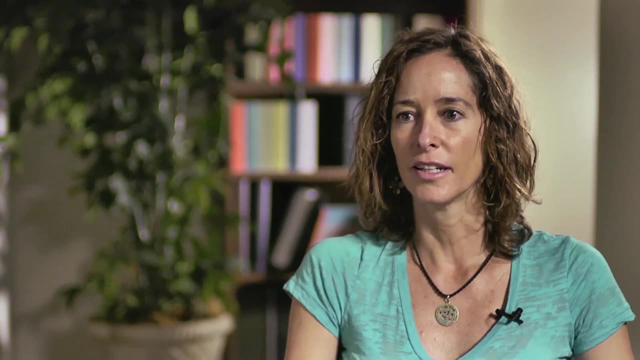 because it's so important to our climate system. You know, I don't think it really was until about 2002, 2003 that we started to really start paying attention to what's happening in the Arctic, Because before that we would have, you know, we'd have low sea ice years in the 1990s. 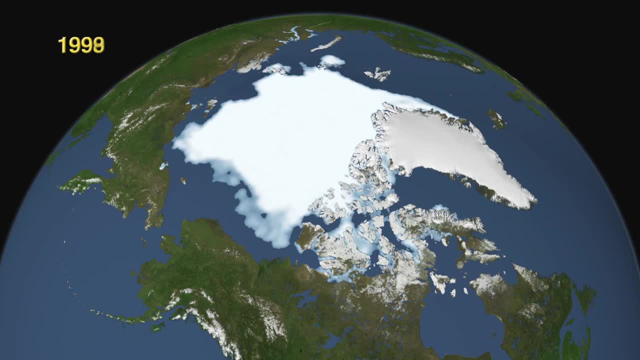 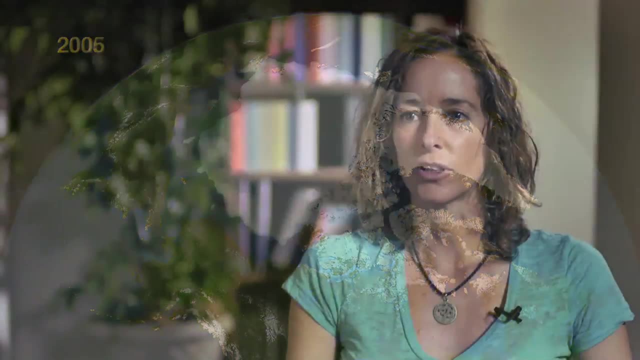 and then they'd be followed by a high sea ice year. But what started happening in the 2000s is you'd have a low sea ice year and then another low sea ice year, and it just kept happening year after year, And that was something we hadn't seen before. 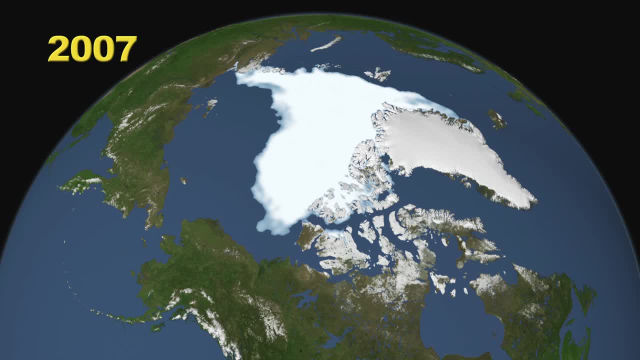 at least during the last sort of 50 years of data collection. And then, when 2007 happened, we had 26% drop from the previous September in 2006, and everybody was like what is going on? Because nobody expected that large of a drop. 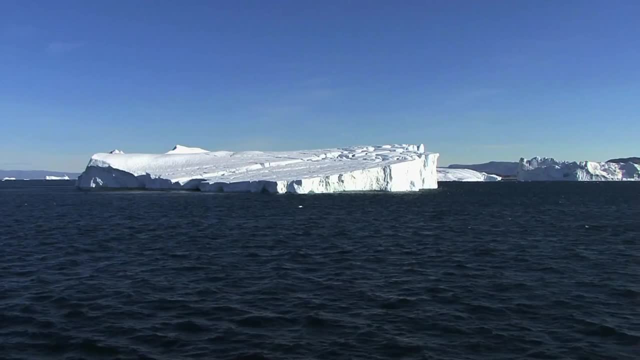 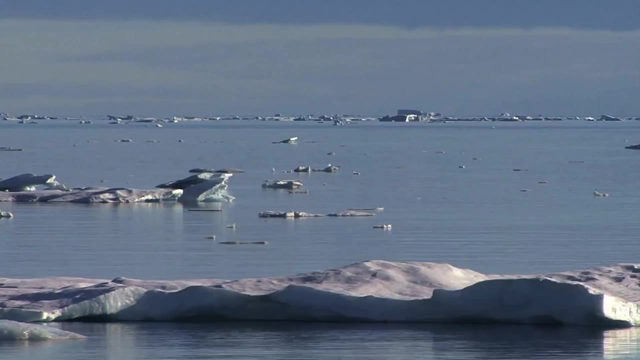 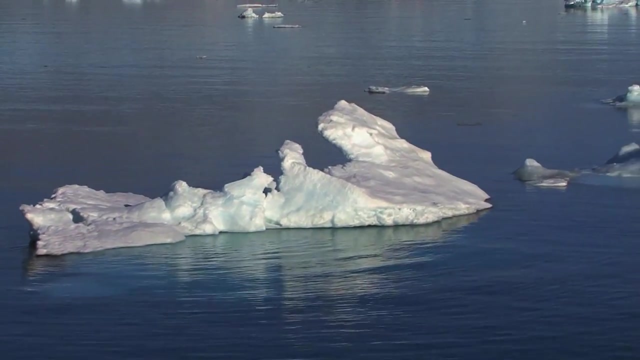 It took everybody by surprise in the science community. The rate of decline right now over the last three decades, is about 14% per decade, And this is actually faster than most of our climate models are actually capturing today. These projections of ice-free dates of like 2050 to sometime beyond 2100,. 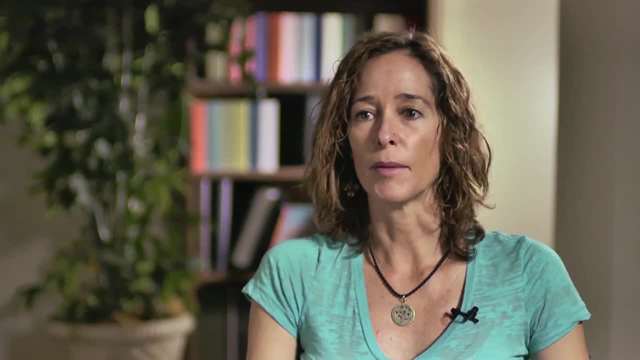 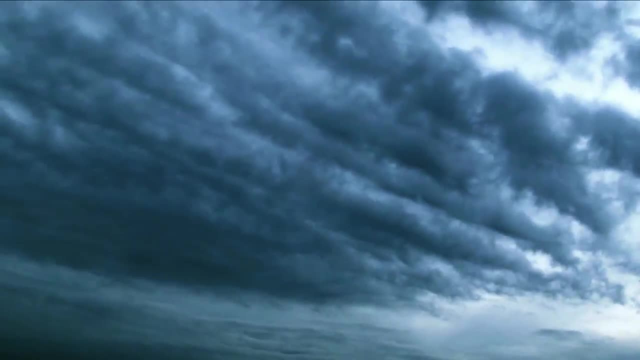 it looks like it could happen a bit sooner, so like 2030.. It might be a more realistic date as to when we might see no sea ice in the summer in the Arctic. You know, basically everything on the planet is connected And the Arctic is sort of the big refrigerator for our planet. 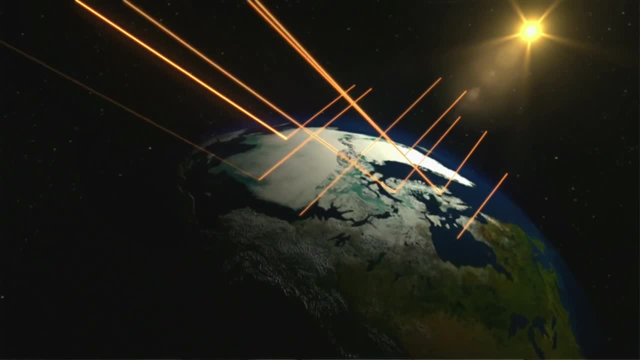 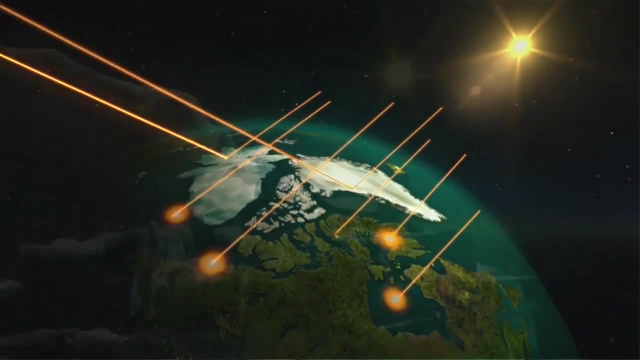 It helps keep our planet a lot cooler because, as you know, snow and ice reflect most of the sun's energy that comes in during the sunlit period. So if you remove the snow and you remove the ice, then the land can absorb that heat from the sun. 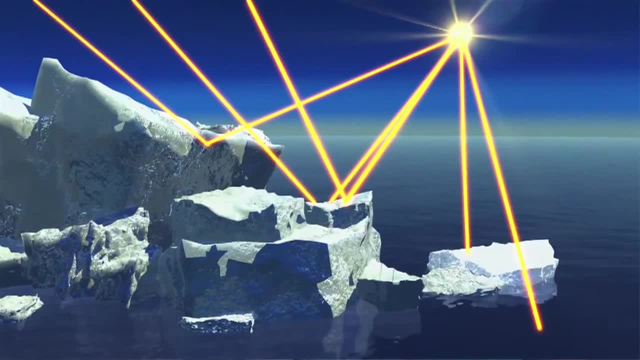 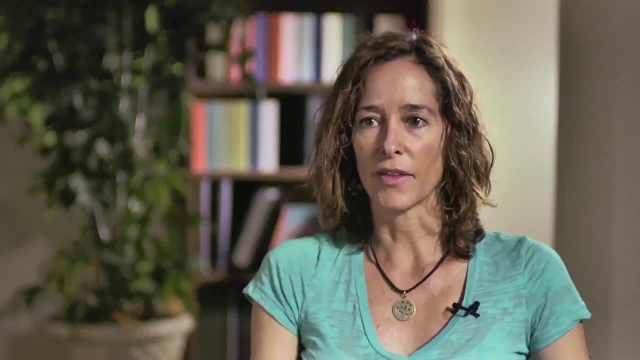 or the ocean can absorb the heat from the sun and warm up further and amplify the warming in the Arctic, for example. All of our weather systems, our large-scale weather patterns, are driven by that temperature difference between the equator, which receives most of the sun's energy. and the polar regions, which receive very little of the sun's energy. But if you change that difference in the temperature between the two regions, you change the speed of the large-scale weather systems that move around the planet As you change the temperature gradient. 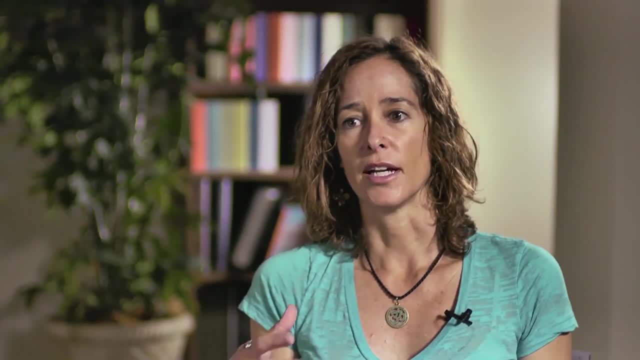 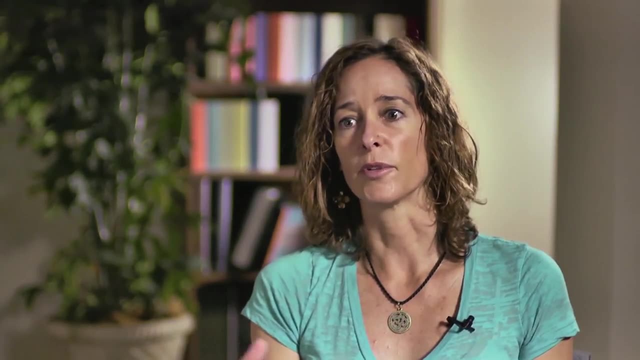 these weather systems start to move more slowly through our atmosphere, And you can get more extreme conditions, such as droughts and floods that just last longer in a particular region, because these weather systems are moving that much slower, And so there is a connection between what happens in the Arctic. 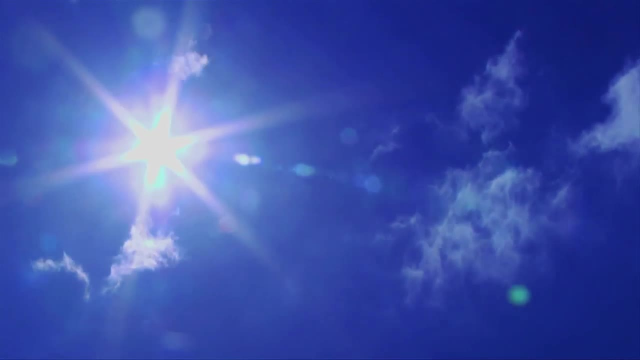 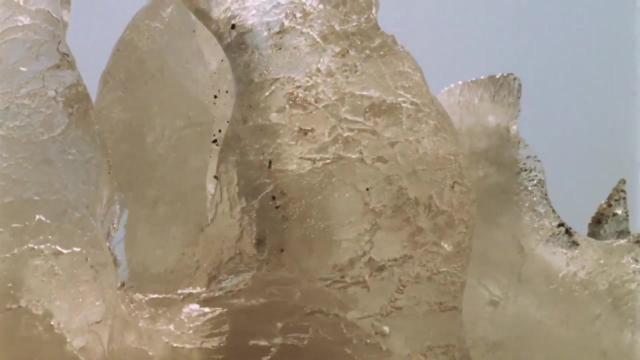 and weather in the lower latitudes, And we knew that if the planet started to warm and you start melting snow and you start melting ice, you're going to have this sort of feedback effect that's going to amplify the warming because you're going to warm up, you're going to melt more snow. 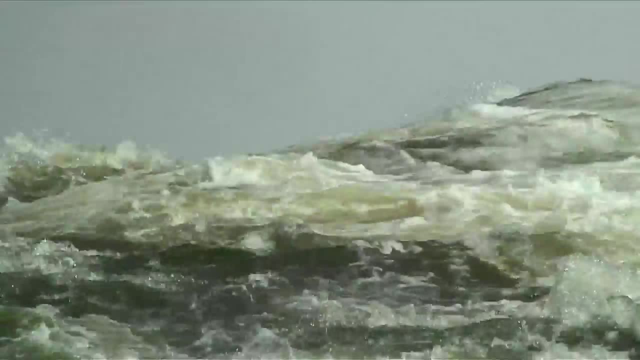 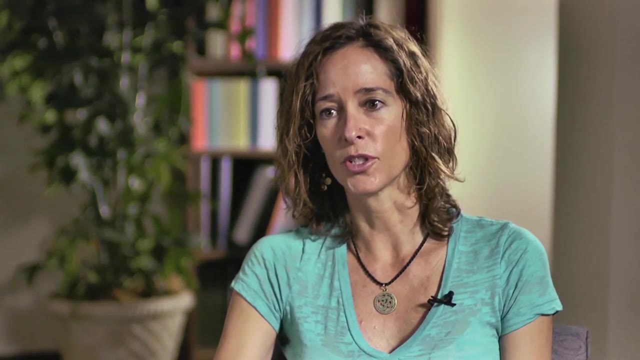 you're going to melt more ice. it's going to further warm everything up and melt more and more snow and ice. so you have this really vicious positive feedback loop. So we knew that the Arctic was very sensitive to increases in temperature And it's responding like you would expect it to. 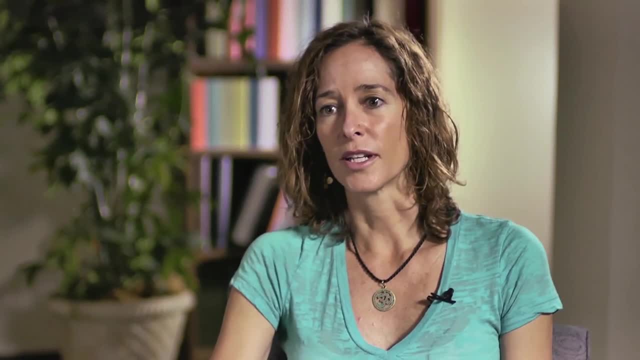 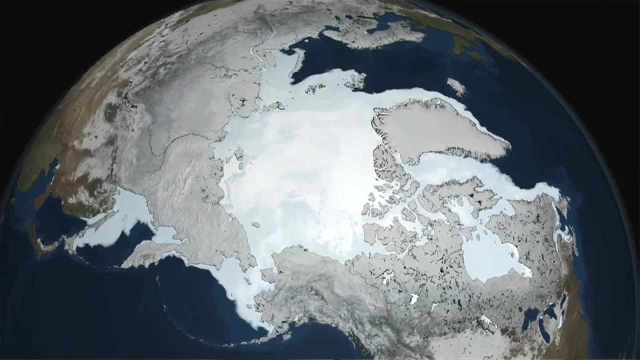 as the temperatures have warmed. So it is sort of our early warning system. We did expect changes to happen first there compared to anywhere else on the planet. We looked at the factors that we tended to use to explain past low sea ice years. 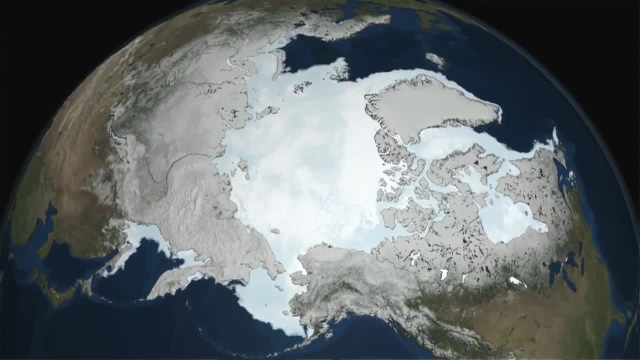 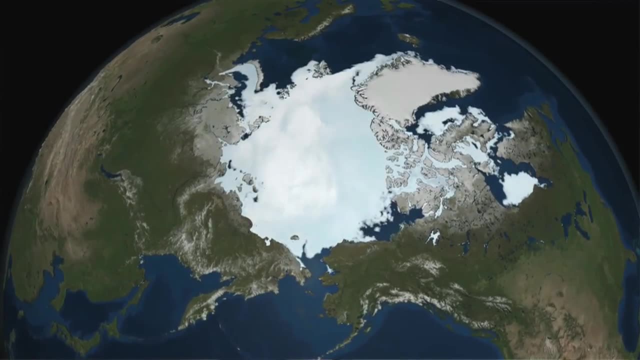 and those factors really weren't working anymore. So it wasn't necessarily a certain weather pattern or a certain temperature pattern that was causing it. There was some sort of background forcing that was happening on the ice cover, that we, you know, were trying to figure out what that was. 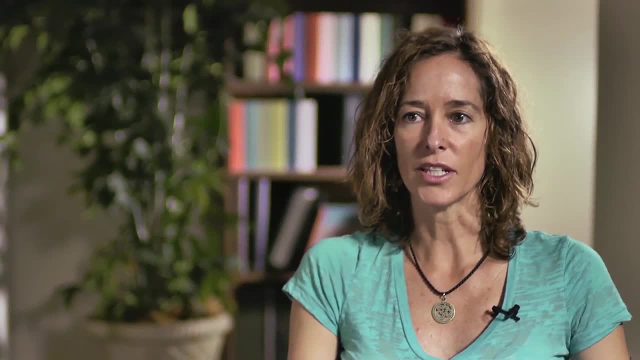 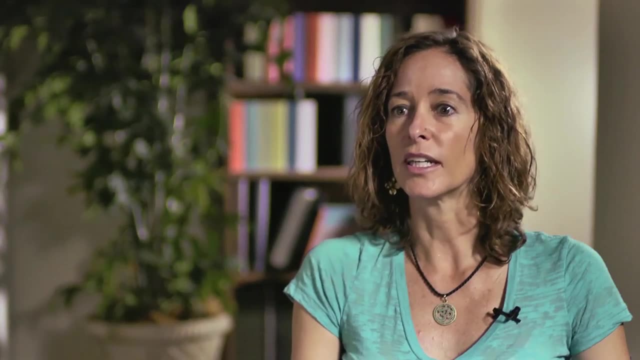 When I started looking at the climate models and comparing them to the observations, then I started realizing: well you know, all of these models would be in their own phase of natural climate variability, so they could be showing increases or decreases over a period of observations. 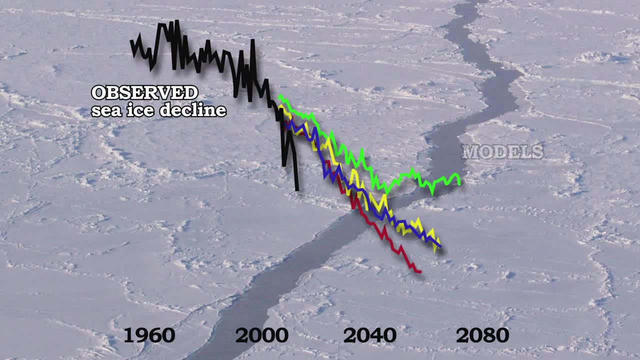 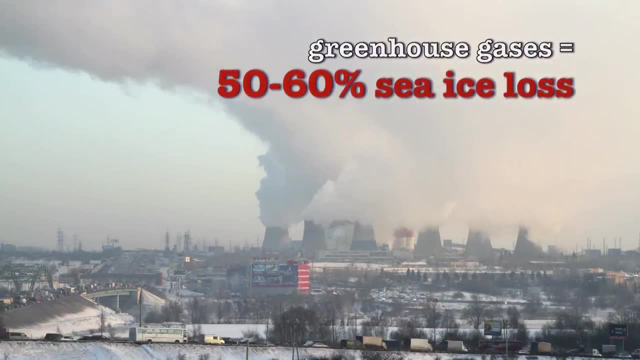 But they're all showing a decrease And so that sort of starts to help implicate greenhouse gases as forcing the changes that we're seeing today in the ice cover. We can say that about 50 to 60 percent of the loss of sea ice that we're seeing today. 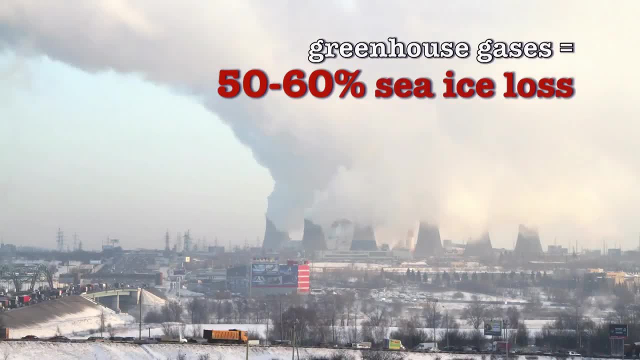 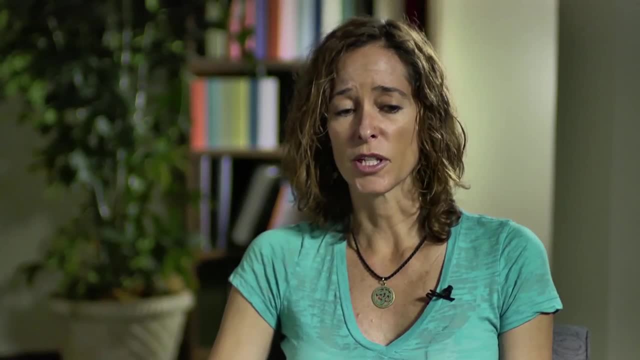 is a result of greenhouse gases. The other 50,- 40 to 50 percent- is actually natural climate variability. So we know both are acting on the system right now And right now the results are about 50-50, I think in what's happening with what we're seeing today. 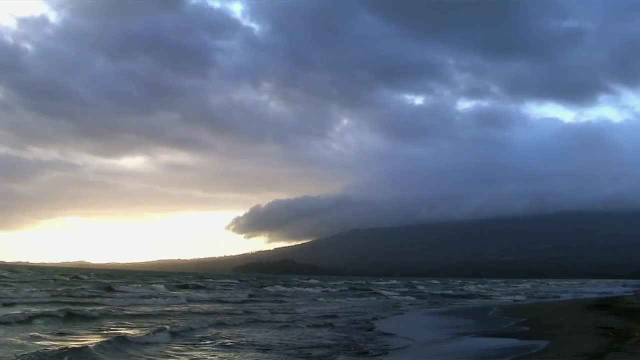 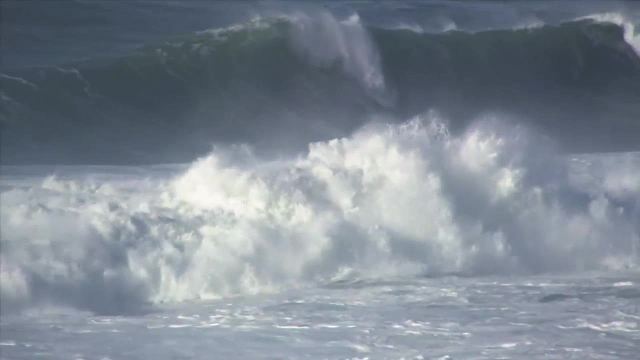 The planet's going to warm by a certain amount of degrees, The sea ice is going to disappear in the summertime. The ice sheets are going to continue to respond, The oil level's going to continue to rise. But when we look at things like